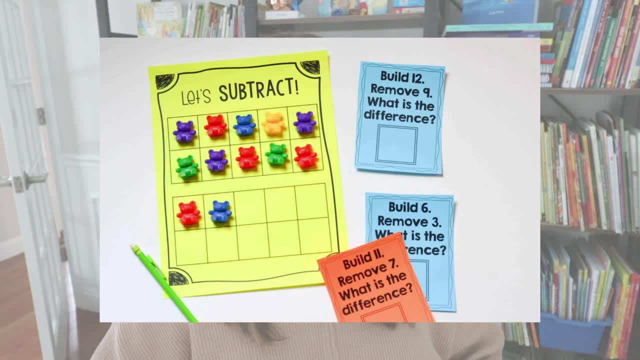 a subtraction unit because students have to actually go ahead and build that 12,. if they are working with numbers over 10, I look for them to fill that 10 frame first and then add the additional two, And then they have to actually physically remove nine of them to figure out what. 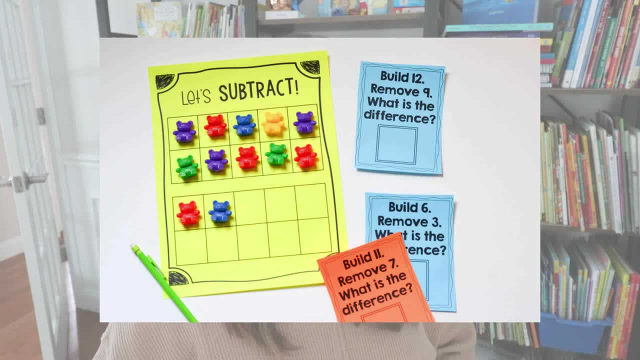 the difference is, and they'll write the difference in that box there Now those colored cards over on the side. I laminate them and the board and then students just use this with a wet erase or a dry erase marker. to be done over and over again. That activity- Build and Remove- is definitely a. 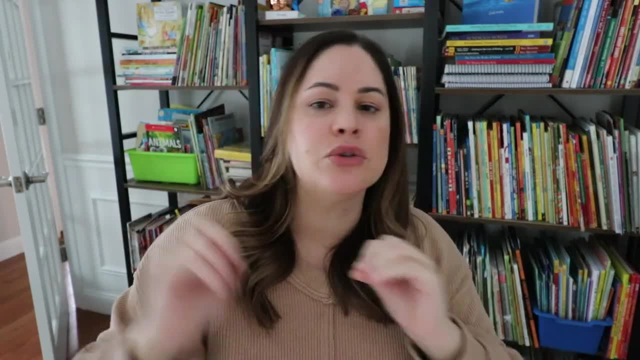 concrete one Again. I want them building a number practicing that one-to-one, and then I want them building a number practicing that one-to-one, and then I want them building a number practicing that one-to-one correspondence or unitizing if the number's over 10. And then they actually have to physically 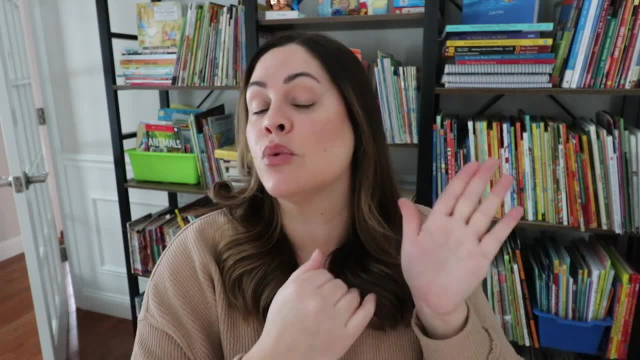 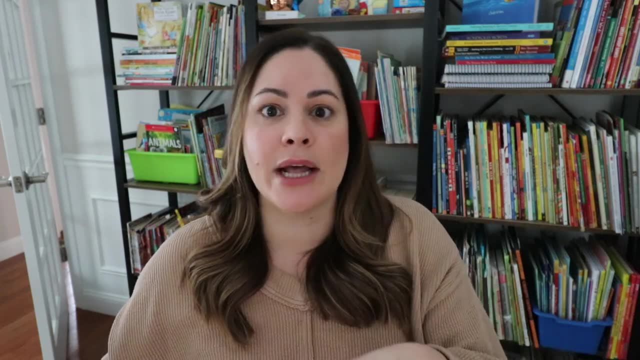 remove to find the difference. I also like that the cards say the word difference on there for a little subtraction vocabulary. And I like this because you can definitely extend this activity as well. After I've had my students do this once or twice, I like to give them either scrap paper: 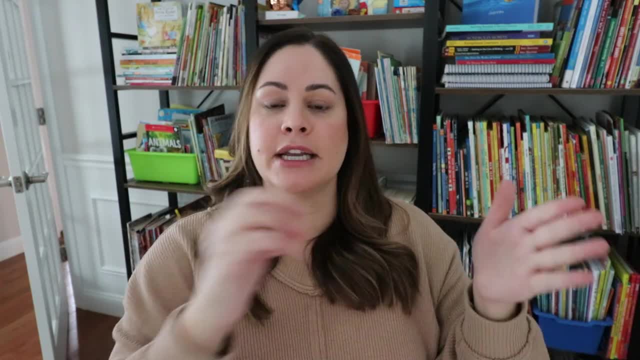 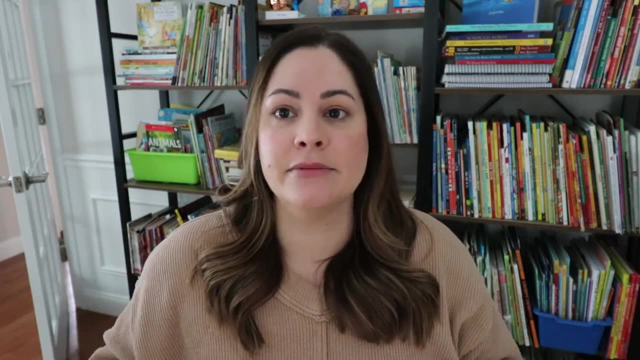 or a whiteboard and marker, And instead of just building, removing and writing the answer in the card, I want them to go ahead and write the subtraction equation. And then I want them to write the subtraction equation underneath it, Or not underneath it, sorry, but on the scrap paper, or 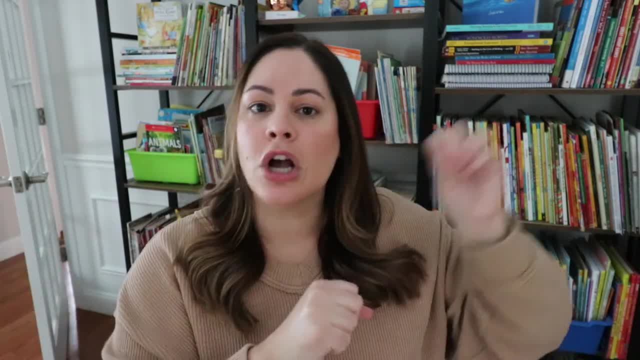 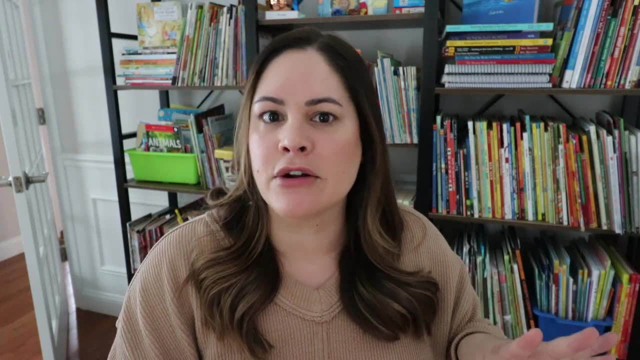 on the whiteboard. So here they are, connecting the actual, physical, concrete with the abstract. They're seeing what that subtraction equation actually looks like, feels like, and then they can figure out the difference. Now that board and those cards are in my subtraction for first grade. 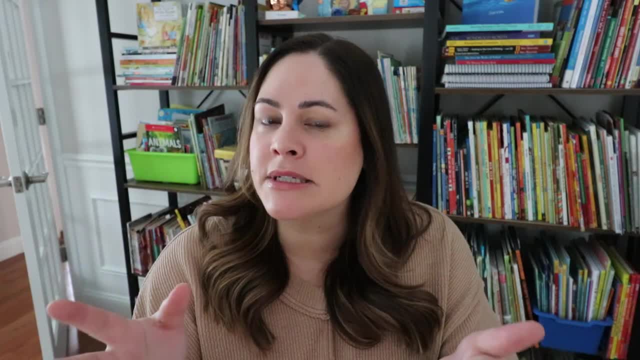 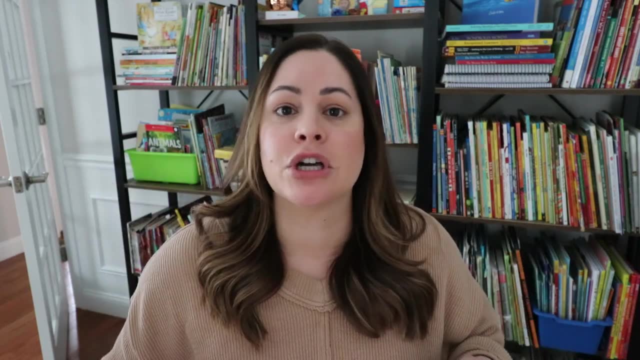 unit. that was done, you know, a million years ago. I hope you can see that it's pretty simple if you want to use it in your classroom. You could just get some 10 frames, have them on the board and then just type up a bunch of cards that say: build 9,, remove 3.. What's the difference? Build- remove. 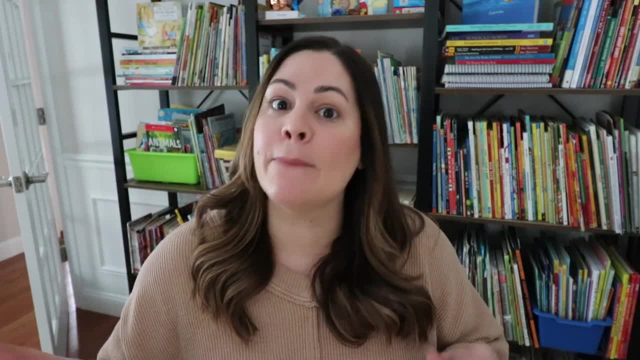 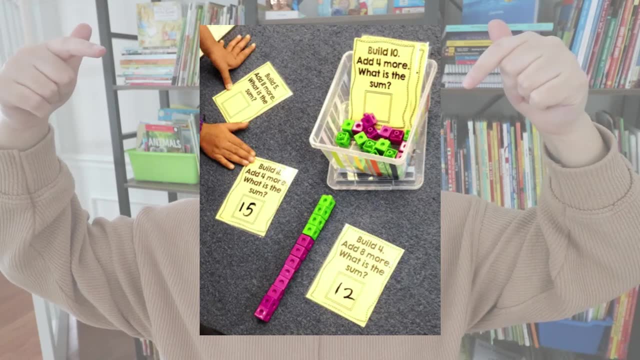 fill in the difference. I had made that as the counterpart to my free build it cards, which are addition based. Here's what these look like And again, these are addition, but these are completely free. over on TPT, where students are doing something similar, Here they go ahead and build. 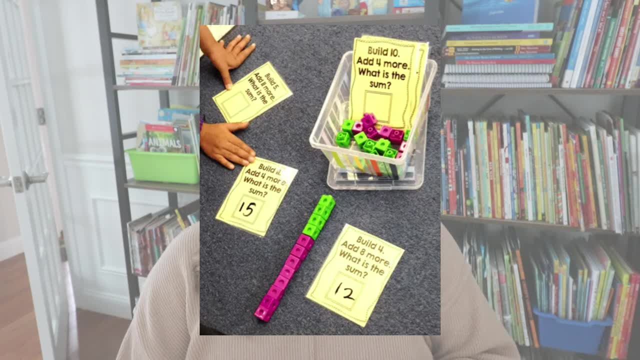 a number using blocks, and then they add a certain amount more. So here we see build 4, add 8 more. What is the sum? And instead of doing this on a tens frame, which again you could definitely use as an extension, 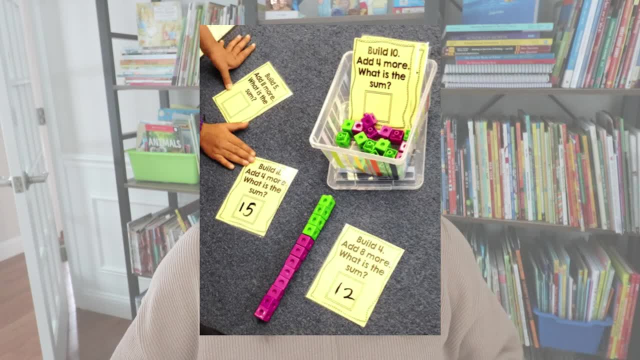 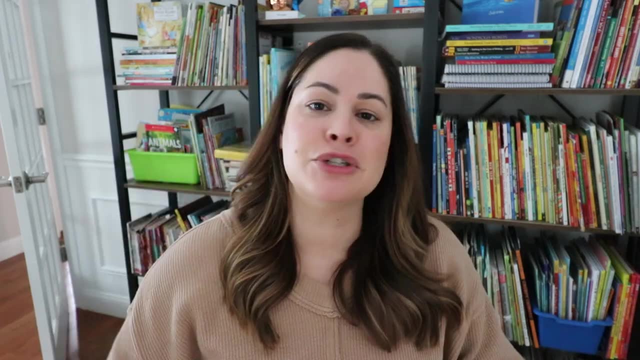 I just have them build it using two different colors so they can clearly see the two parts as they make that whole. I know this is a subtraction video, but I'll link that freebie down in the description for you as well. All right, Subtraction game number two is a class favorite. This is a. 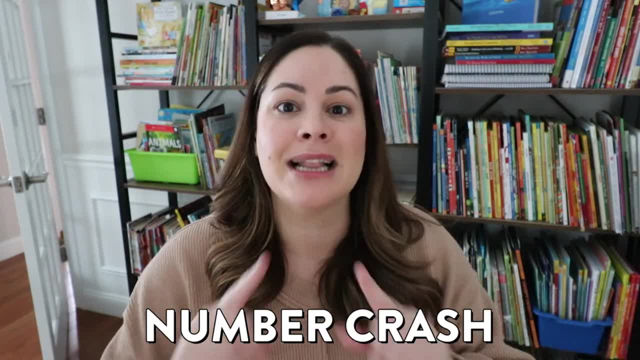 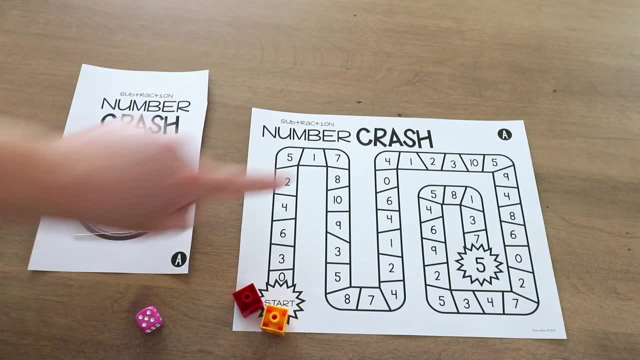 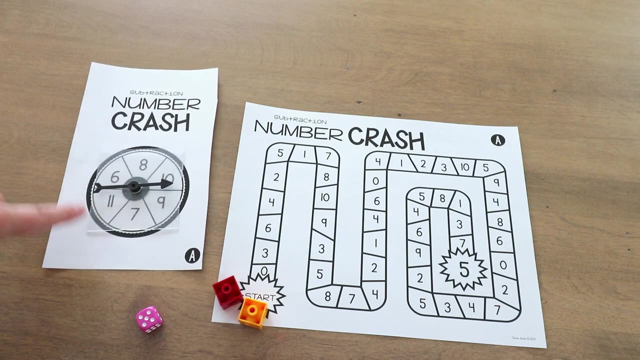 print in play game and it is called Number Crash. Let me show you how this works. All right, This game is called Number Crash. There are two different versions of this game. We have the differences within, or subtraction within, 11.. Actually, it's going to be the highest number And then the other. 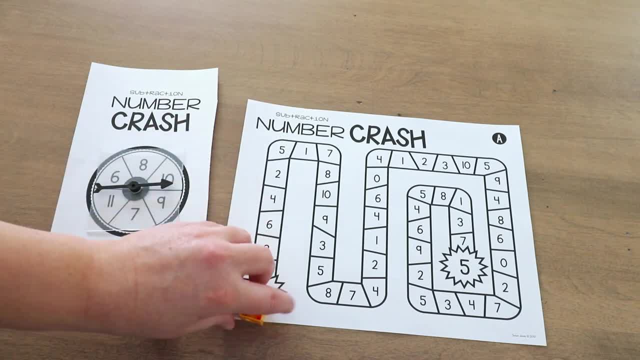 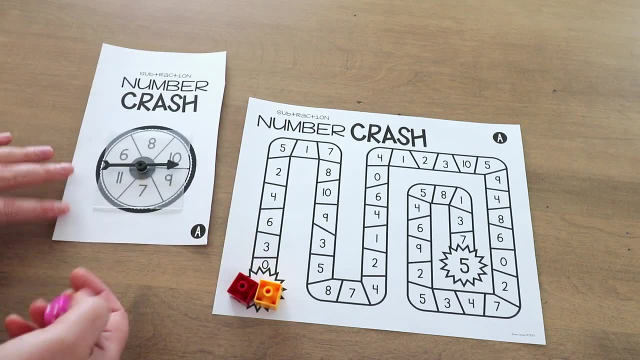 version goes up to 20.. So there are two different game boards for you. But this is a partner game, So students will each have their own little game cube and they start on start And they will have to do two things. They will spin the 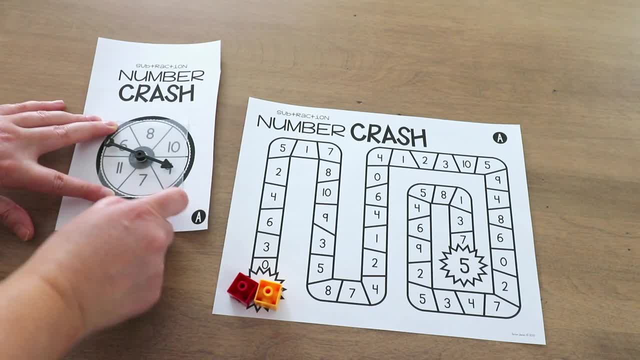 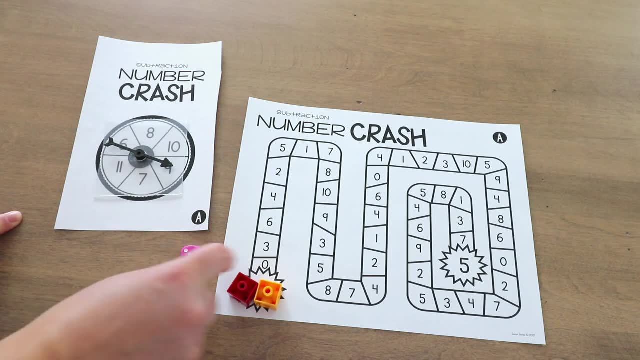 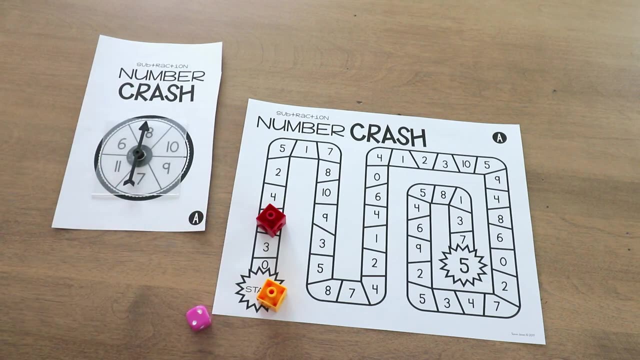 spinner nine and they will roll the die. They'll always do the spinner minus the die. So we have nine minus three. That difference is six. So I will move to the closest difference here. Player two will go eight minus two. Eight minus two is also six, Since this is the first one we actually 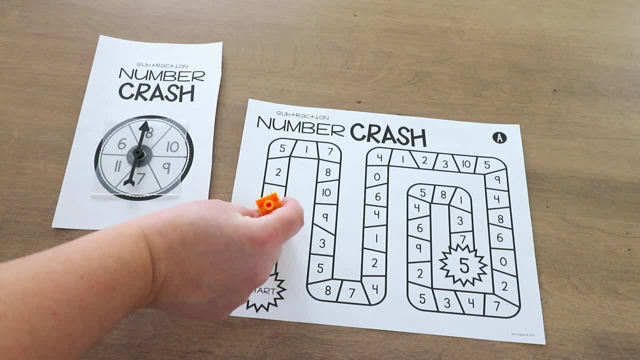 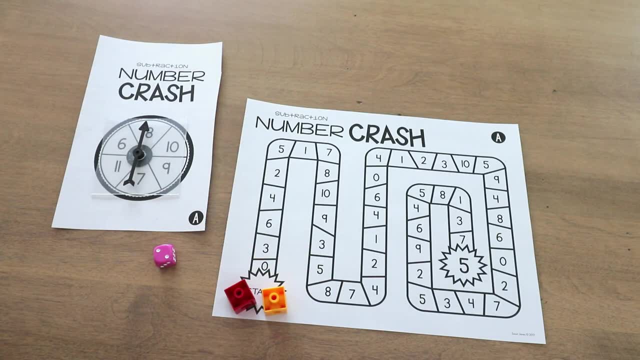 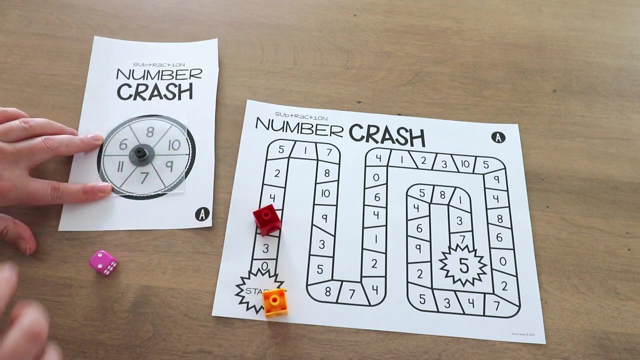 already have our crash. Whenever students happen to land on the same number, the same difference, they crash and have to both go back to start. So then we go again. Eight minus two. Oh my goodness, Here we go Six. See if we get something else. 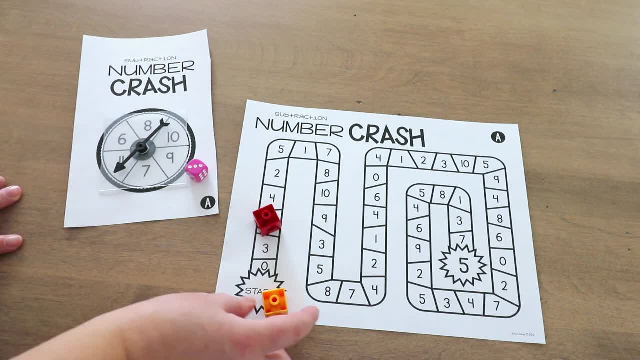 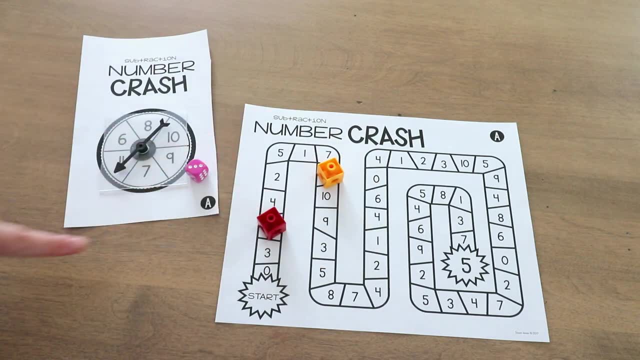 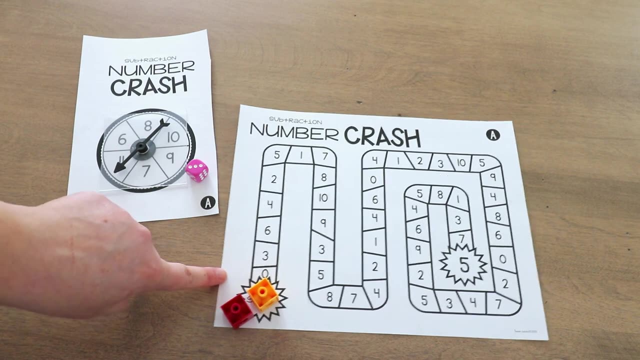 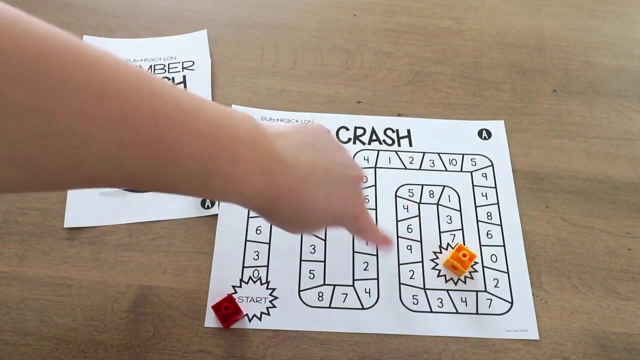 Eleven minus three. Eleven minus three is eight. This player gets to go all the way to the first difference of eight And students just go back and forth, But every time again they land on that same number, they crash and they both get sent back to zero. the winner will be the first player to make it to the end, which is going to be a difference of five. So whoever can make it there first without getting crashed wins the game. Now, the way the game is set up, there does happen to be a lot of crashes. We're still in the middle of the Kafaro. 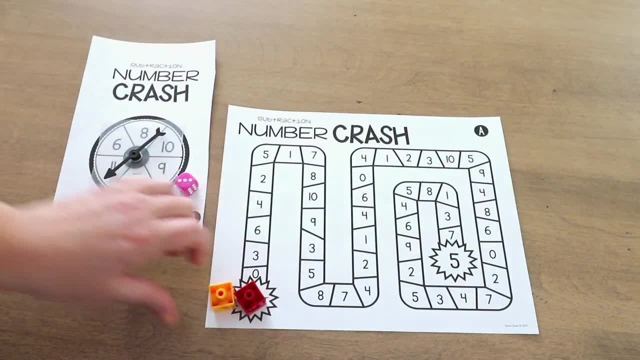 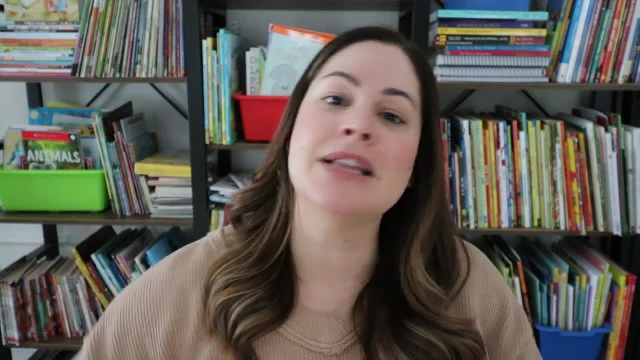 which is a good thing, because then they are, you know, forced to go back to the beginning and practice that fluency again. right, They have to keep spinning and subtracting and moving. Subtraction game number three that I love is called Fill the Spaces. Now, this is another. 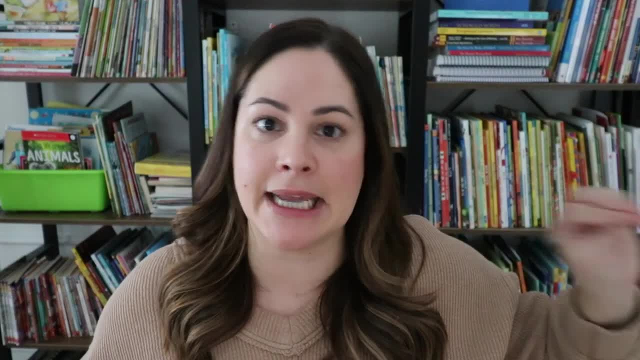 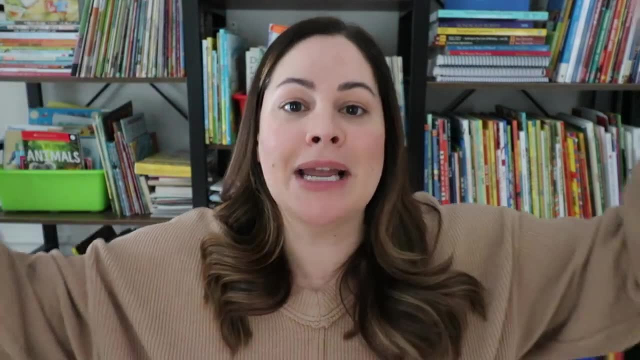 print and play game, just like Number Crash. It actually comes from the same unit. This one I have available for free for you, though, so I'll put that as a freebie linked down in the description, But here is a picture of what this looks like Now. this is a very simple game that I like using. 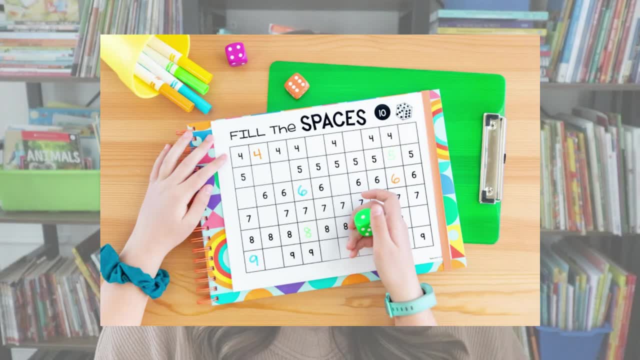 to help develop fluency with subtraction. but basically the board looks like this: right here It'll say Fill the Spaces at the top and it has a little 10 up there with a die next to it. Now you can see that there are some empty spaces in the board and the goal of the game is to fill. 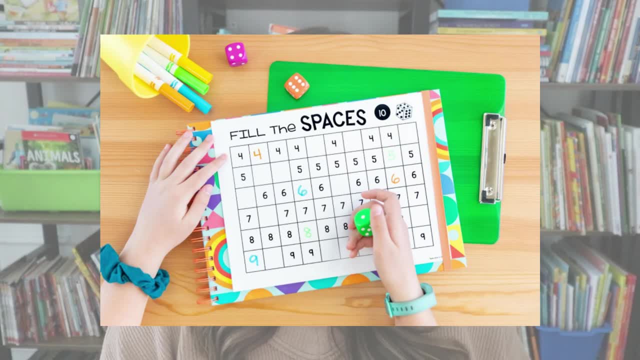 the spaces, hence the title of the game. All students need to play this game is one die, the game board, and then two different colored crayons or colored pencils, And all students will do is take turns rolling the die, and that is the end of the game. So if you have any questions, 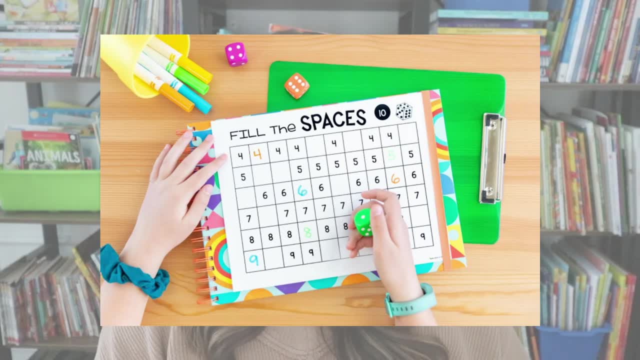 please let me know in the comments. And if you have any questions, please let me know in the comments. going to be the number they subtract from 10.. That's why the 10 is up there. This is going to be fluency with subtraction within 10, so students can hopefully quickly start recognizing these. 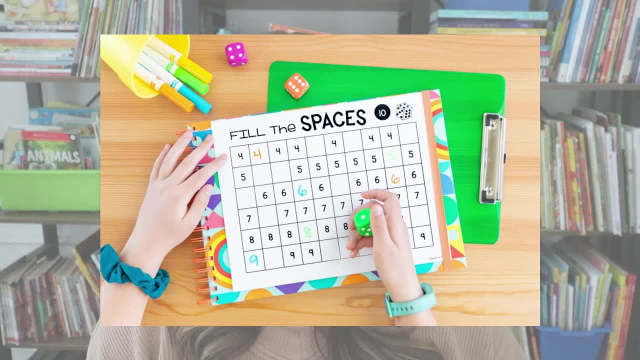 differences. So if they roll a 3,, 10 minus 3 equals 7, and whoever's turn it is will take their colored pencil and fill in one of the blanks or one of the spaces in that row of 7.. Then the 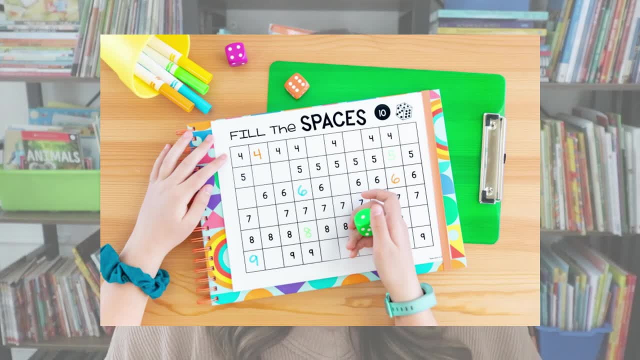 next student will go ahead and roll that die and repeat the process. So if they roll a 6, they will do 10 minus 6 equals 4, and they will take their colored pencil and fill in the space in that row of 4.. Students just take turns rolling, subtracting and filling the spaces until 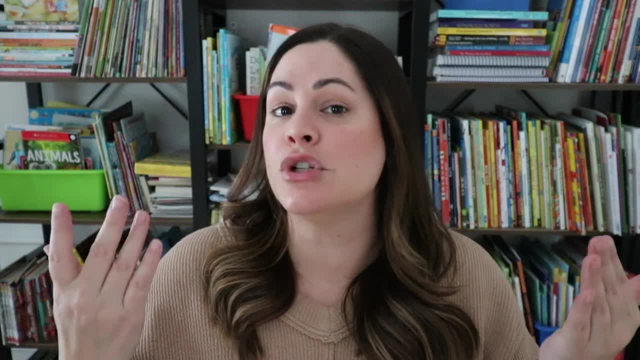 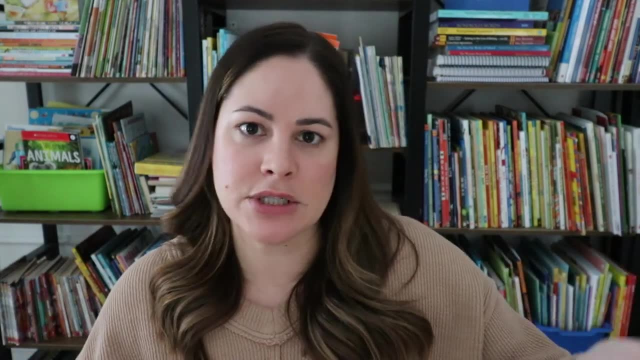 they are all filled in. Now the game part comes in when, if students roll the die and that difference is no longer available on the board, then their turn is skipped and it gets passed to the next person. So they will continue back and forth until the whole board is filled in And then at 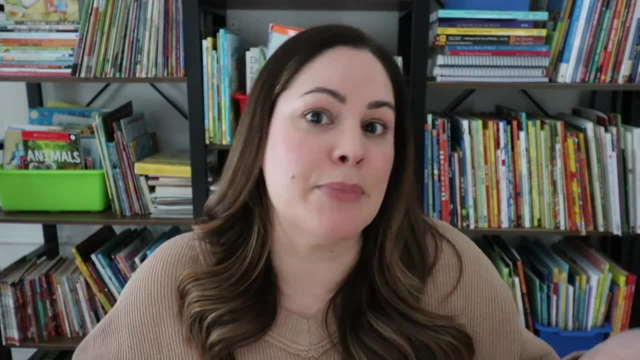 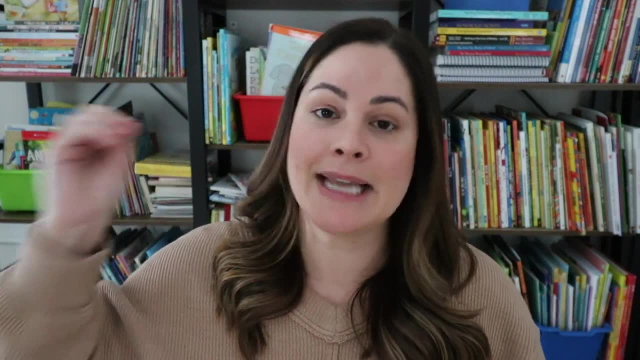 the end, they count up their color and see who got the most, and that person is the winner. Now, while I developed that game for fluency, meaning I want my students to quickly be able to subtract that number from 10, you could definitely add manipulatives as needed for 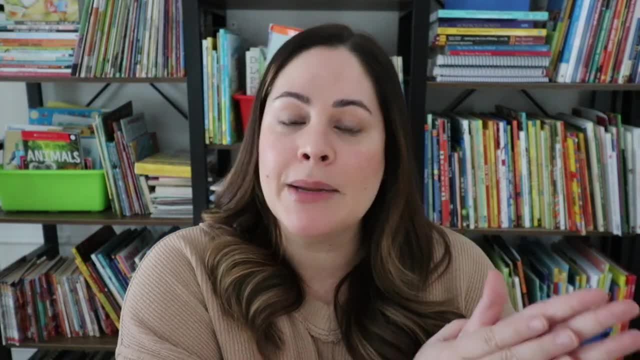 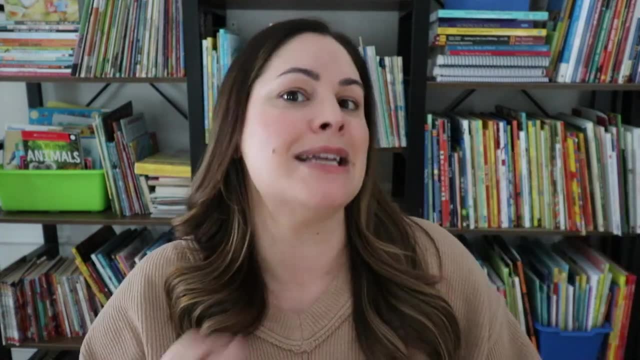 your students. You always want to give them either a piece of scrap paper if they need it or, like I said, cubes, manipulatives, something like that, And the goal of that would be able to slowly take those away as they no longer need it. Alright, math game number four that I love to use. 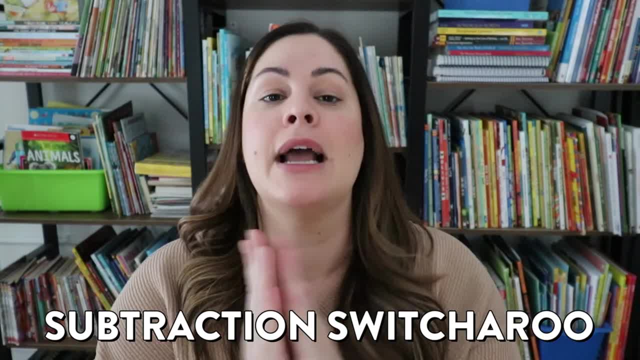 with my students is called Subtraction Switcheroo. Now, this is one of my math mysteries that I came out with. I'm going to show you how to do that. So let's get started. So I'm going to start with. 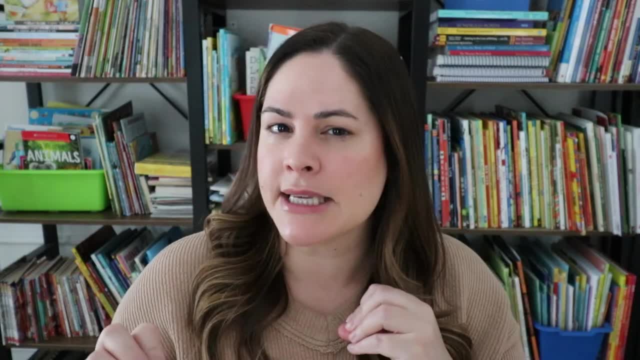 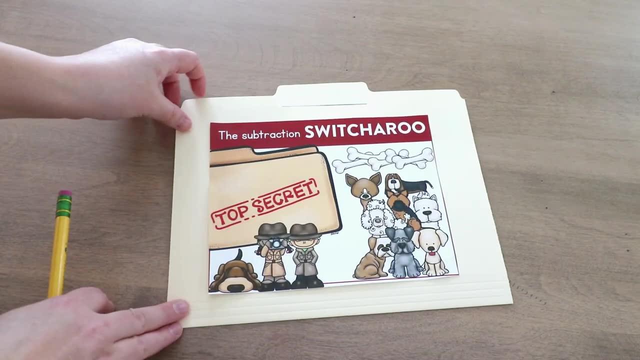 last year. I think I have about seven of them for different skills, but this is the subtraction one. Let me show you how it works. Alright, for the subtraction switcheroo. I store each one in a file folder with the cover. So again, this is subtraction within 20.. And then each one. 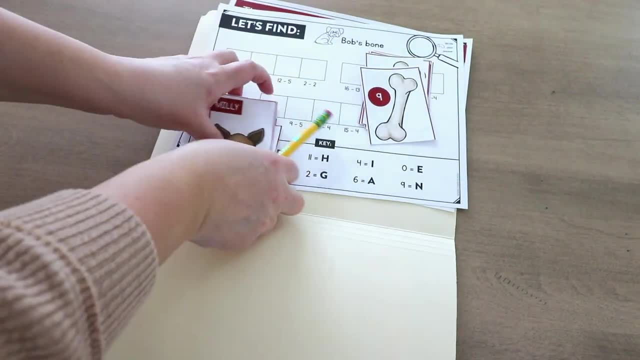 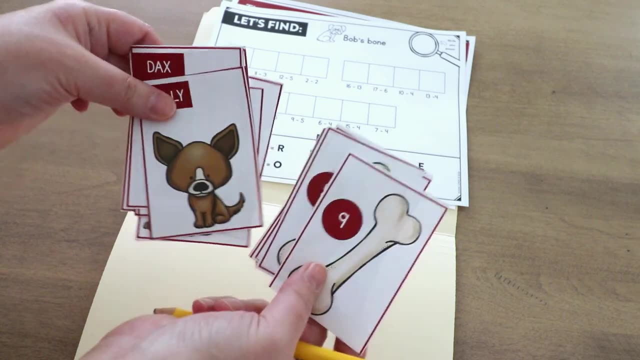 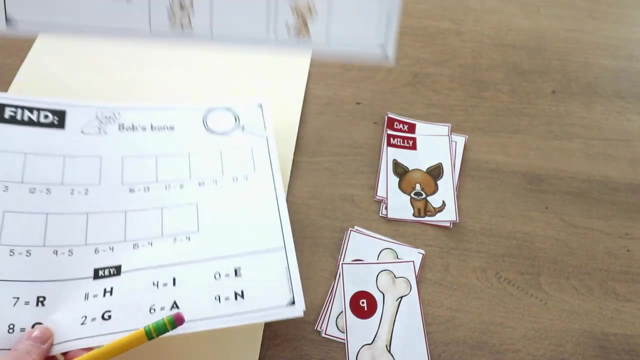 I usually store these in a Ziploc bag, but just to make it faster and easier, This one has eight dogs and eight bones that need to get matched up. It also has eight different clues that look like this. They each say whose bone you're trying to find at the top, And then there is an answer key. 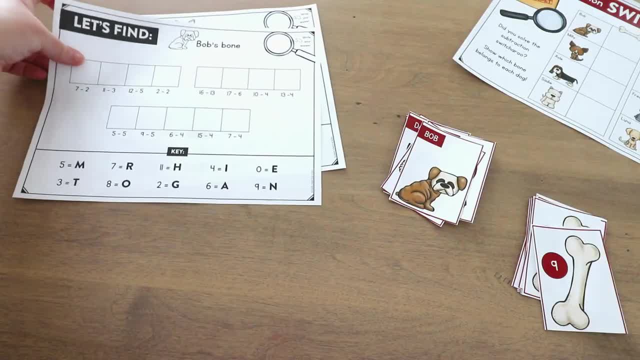 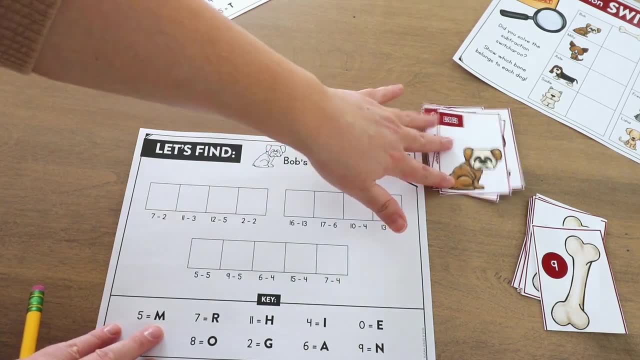 here to kind of show the final product. Once students have all the materials that will be in their file folder, they can go ahead and get started. Now, each one has its own premise. Like I said, here we have bones and we have dogs, And for this mystery that you're trying to solve, 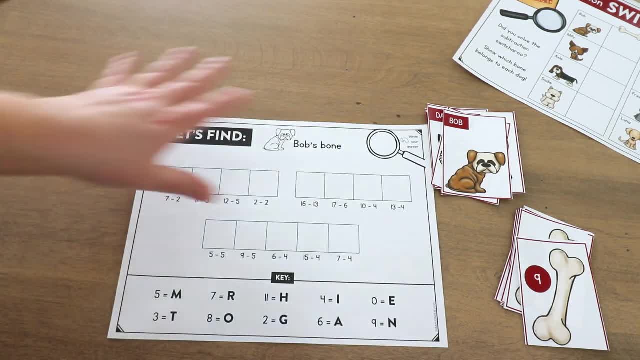 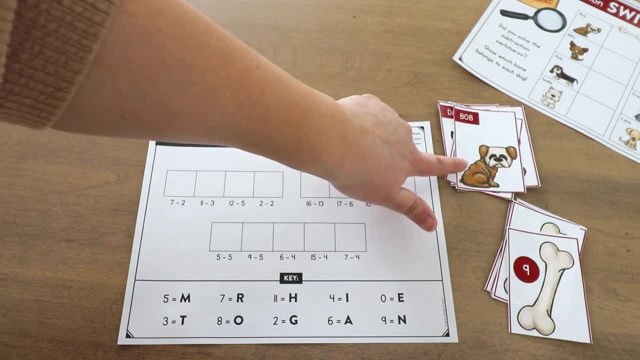 or that students are trying to solve. somebody stole all of the dog's bones and they hid them around the park And you have to find which bone that each of you have to find. Each of a number belongs to which dog. So that is the subtraction theme. And in order to do that, 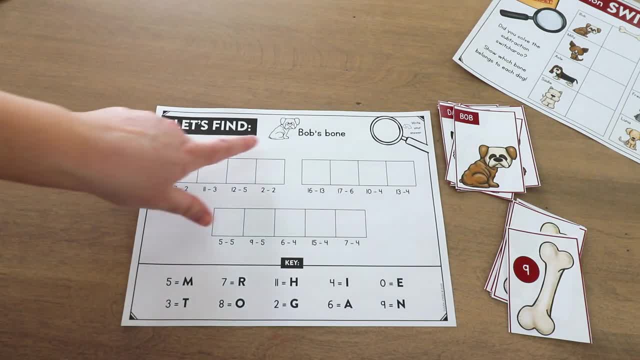 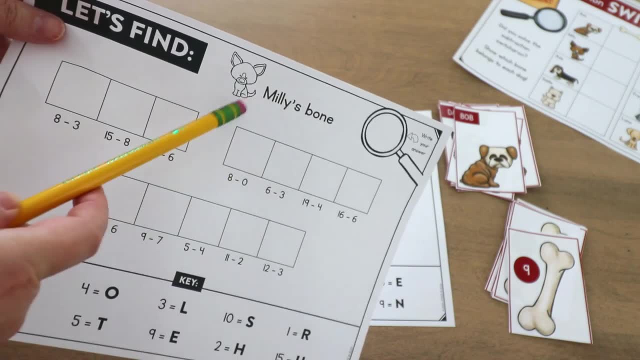 students will have to figure out these clues. So here we can see, we're going to find out Bob's bone. Remember, each one at the top will have the picture of the dog and they will have its name and they'll have that. That's the clue. So here we have Bob and we're going to find out which. 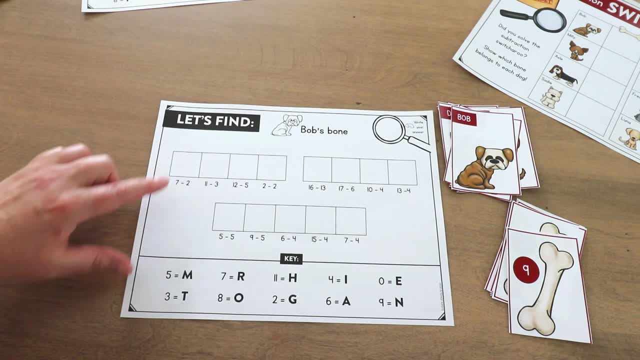 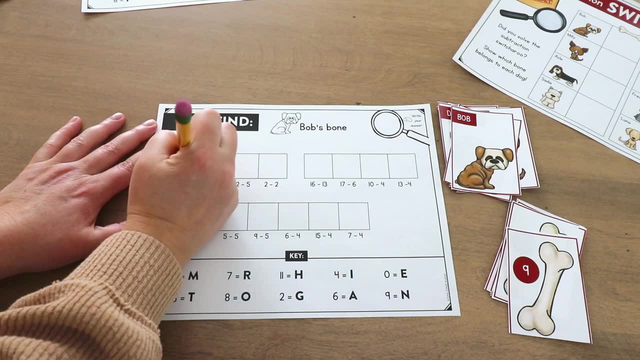 bone is his. To do that, they need to go ahead and solve these clues. So we have seven minus two. seven minus two is five, And then they go to the key. five is M. Eleven minus three is eight O. 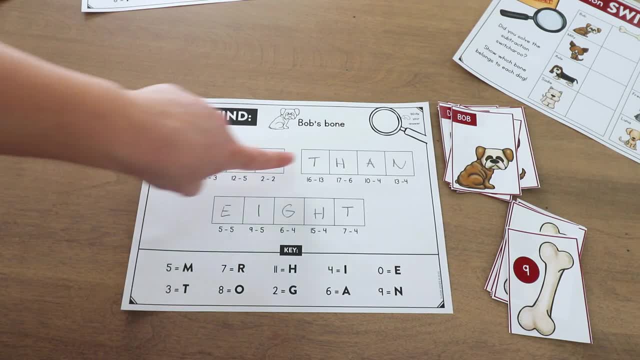 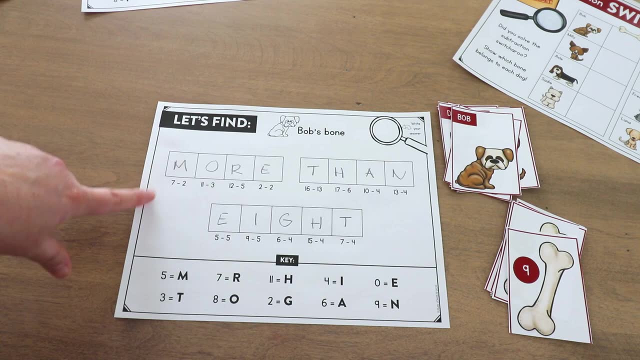 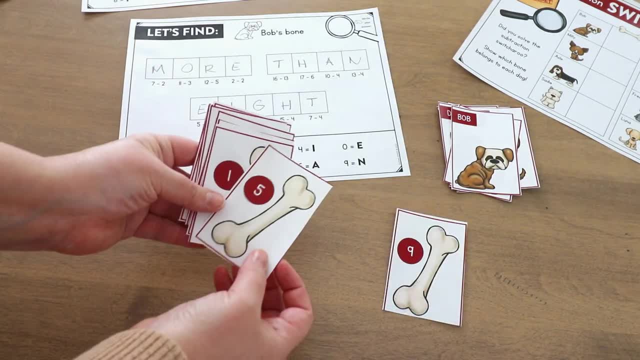 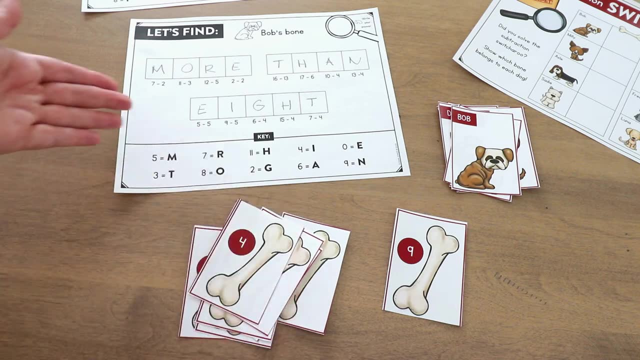 So I'm going to assume that's it And I did not do that on purpose. But you will look at all the clues and students can work together in their group: five, one, six, seven, three, two and four. There's only one that matches that criteria, So Bob's bone must be nine. They can write their. 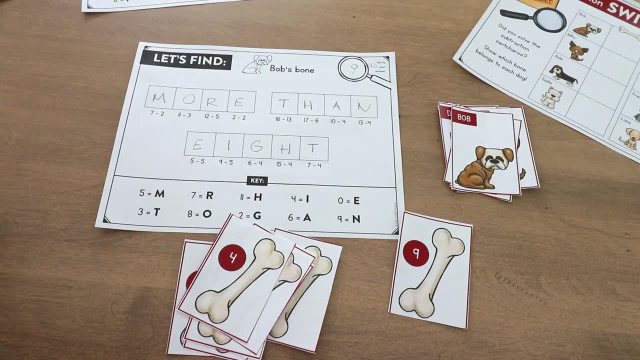 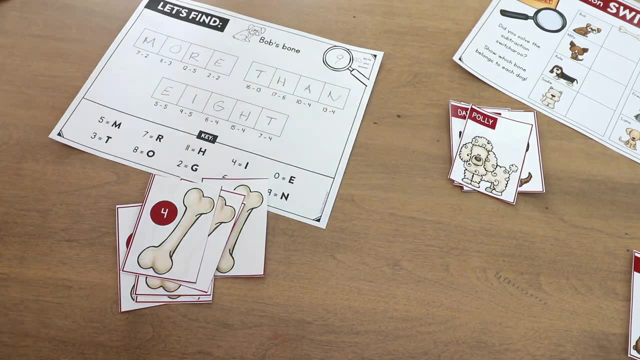 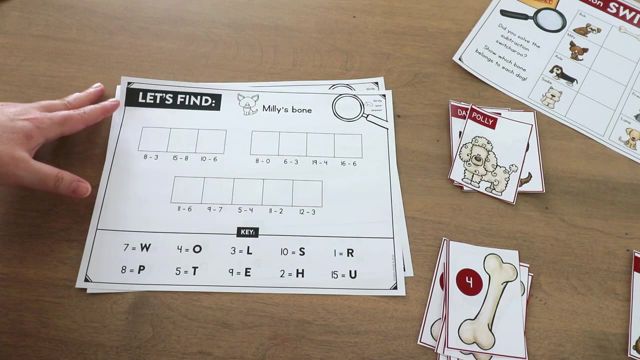 answer right up here. Bob's bone is nine And then I like to have students actually physically take the bones, match them up and move it to the side. Then they can go ahead and solve another clue, Milly's bone. Now, when doing these I would work in a group and I would probably have students work. 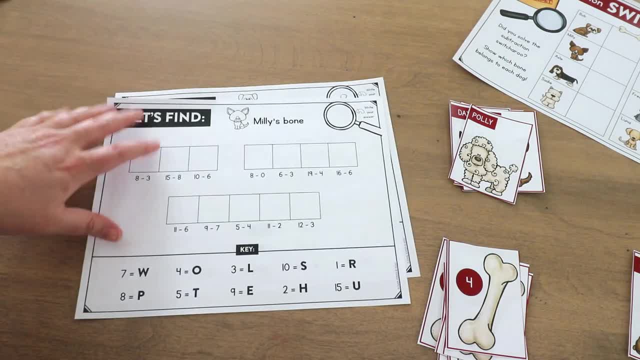 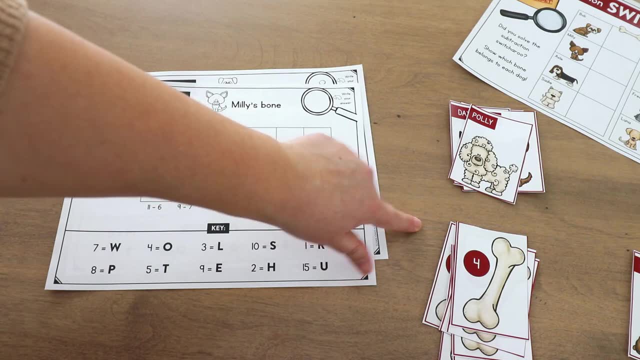 in pairs of three or four And there are eight different clues. So they can divvy up the clues and have them solve and match each one That way as they're solving and matching. if for some reason at the end they think two different dogs have the bone four, they can look at those clues. 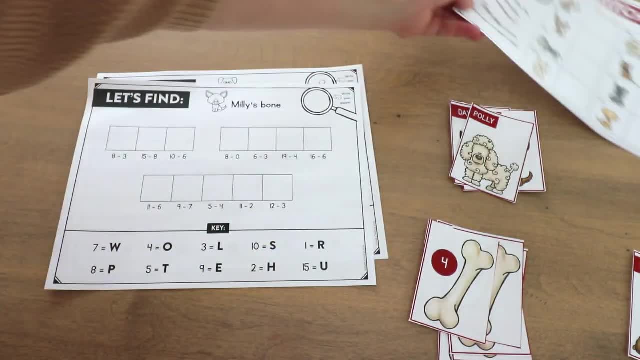 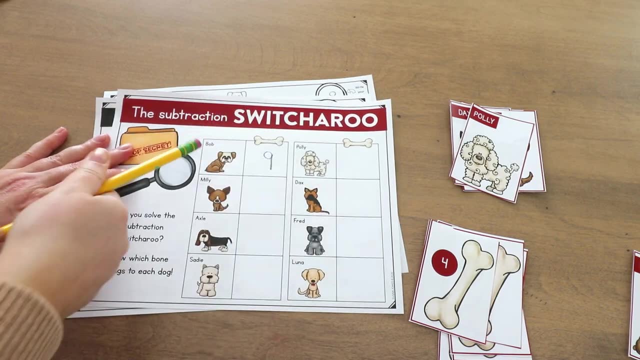 kind of dissect: what's wrong and figure it out. Then, when the entire group thinks that they are completely ready, they will fill in the answer key here And then they can go ahead and solve. so, Bob, we know his bone nine. And then, as they solve the rest, they can fill it in. 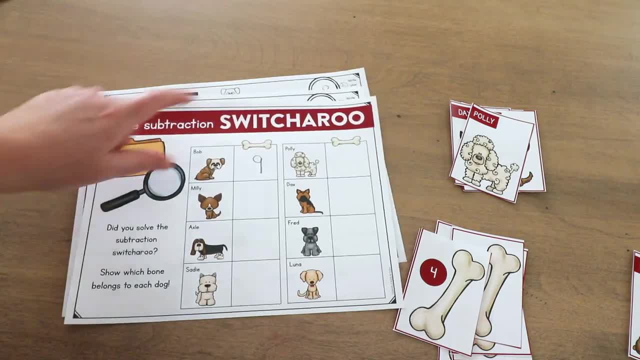 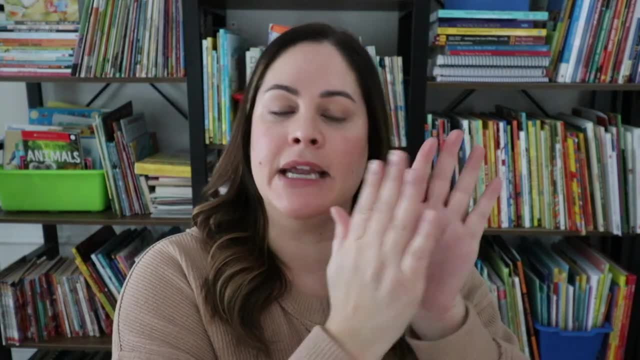 and they can pass it in and say: here we go, We solved the subtraction switcheroo. So I just showed you the hands-on version, which is how I would do this mostly with my students. I store them in Manila folders. They kind of work together to solve the clues. 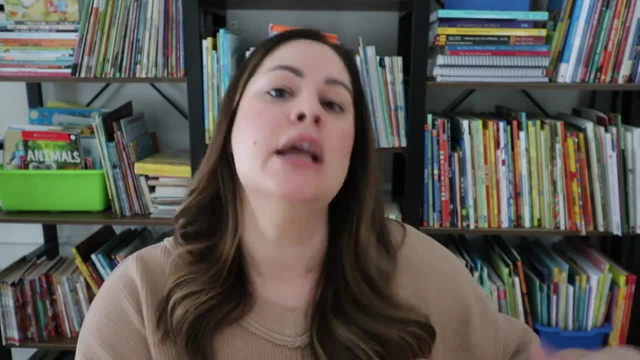 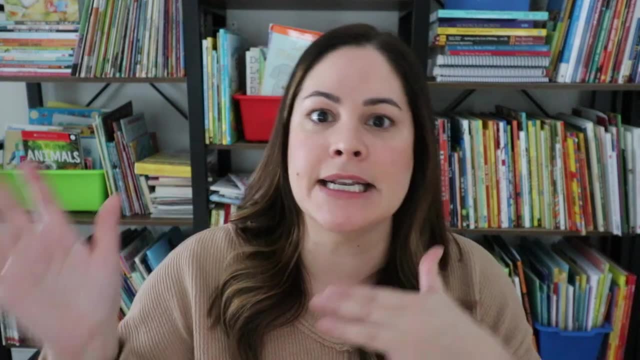 Um, and I would probably do this in one math period so they can practice that, But then I do also have all of my math mysteries available in Google slides and Seesaw If you wanted to make it an independent Activity as well. for the sake of time, I won't go into exactly how that works. 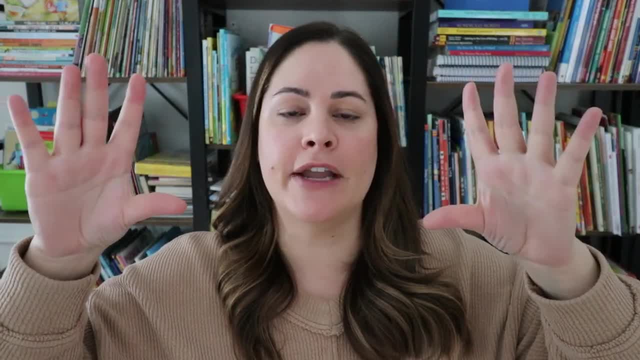 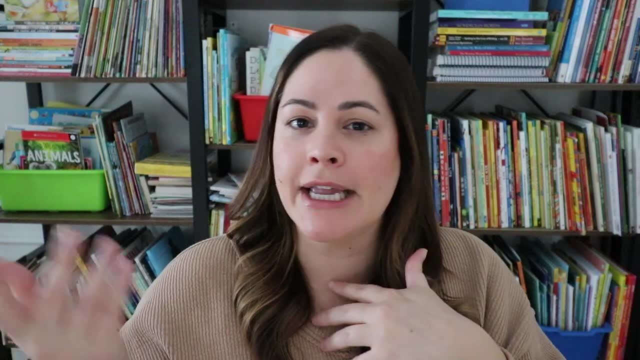 but essentially, since it's independent, I do have a slide on there for students to like put a star over the clues that they already solved, because they probably wouldn't be able to solve all eight clues in one time period or one class period. So I do have something in there for them to keep. 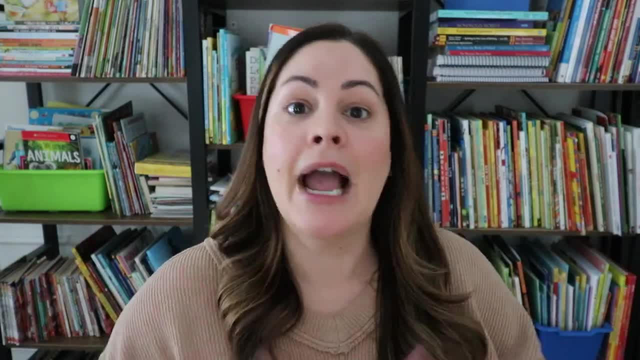 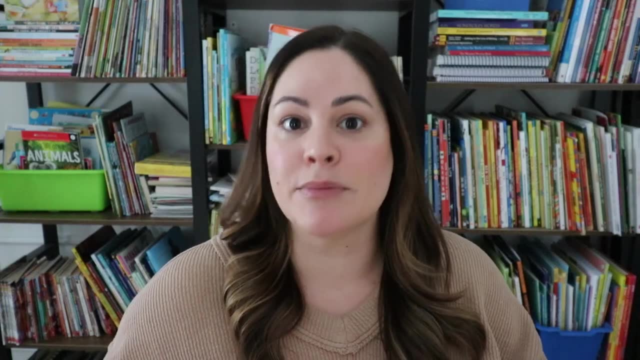 track of the clues they already solved before finishing the whole mystery. I actually just got back from a conference I presented at in Charlotte and at the end of our second and third grade session we did a Double digit addition and subtraction mystery. and they are just so much fun. 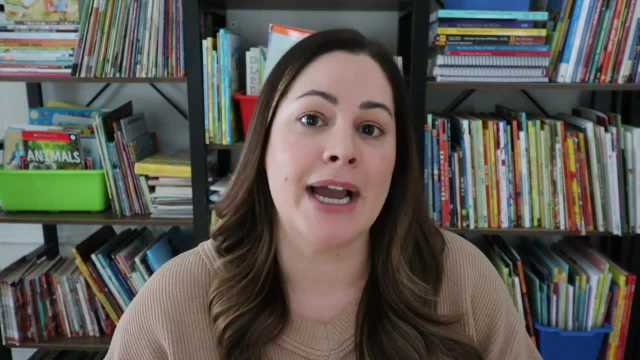 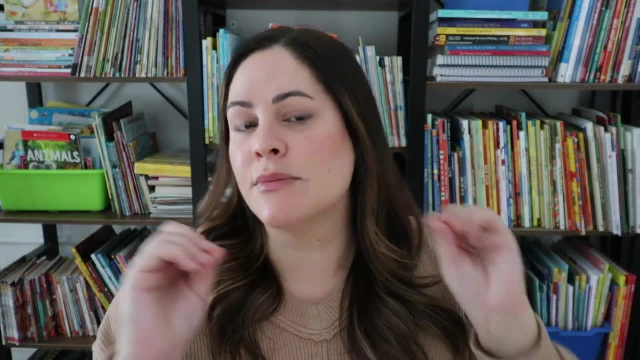 The teachers had just as much fun as the kids did, And I got a lot of feedback saying that their kids would love activities like that. So I will actually link all the math mysteries down below. but this one specifically was called subtraction switcheroo and it was with subtraction. 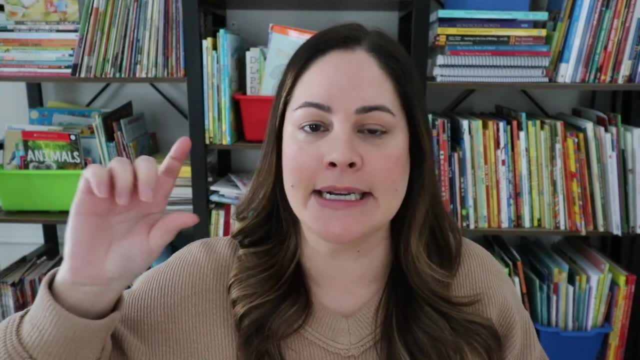 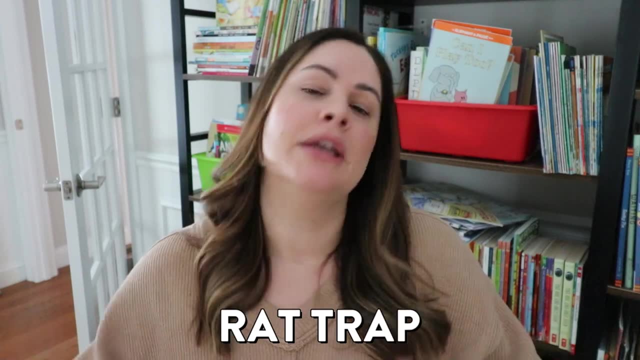 within 20.. So I'll list the category, but then you can find that specific one for your students. and subtraction game Number five that I love to use with my students is called rat trap. Now this is going to be another print and play game that you can again have students use manipulatives if 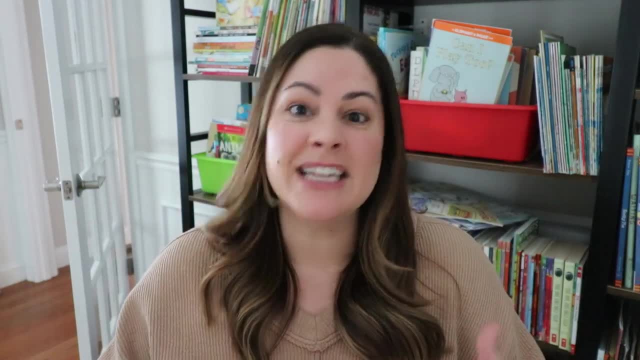 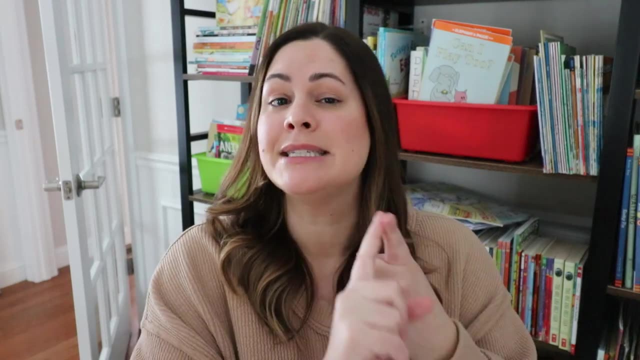 they need it, have them use scrap paper as they need it or, if they are ready, they can do this with subtraction strategies they already know in their head. Now, before I show you what this looks like, I have a version for subtraction within 10,, within 20,, within 50, within 100 and within 1000. 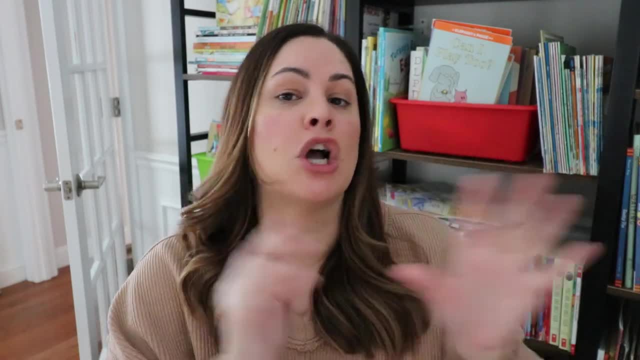 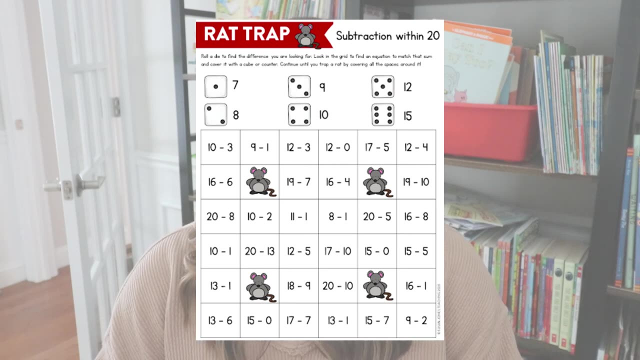 So your freebie for this one. there's actually five different boards based on your students needs, So let me show you what it looks like. Here's the game board. This is the subtraction within 20 which you can see in the top right corner. Um, if it's within 10,, 50, whatever it is. 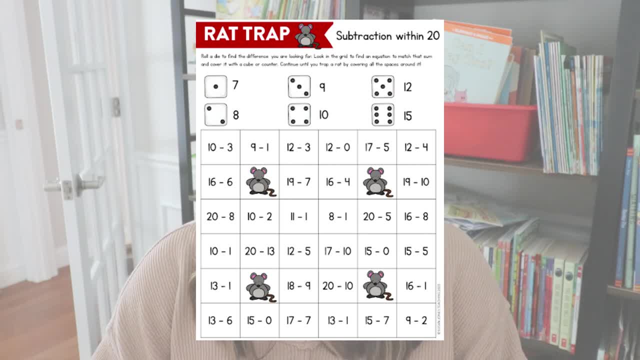 will be listed up there, but students will basically take turns rolling a die to find the difference they are looking for in the grid. So if students roll a one, they are looking for an equation with a difference of seven. If they roll a five, they are looking for a difference. 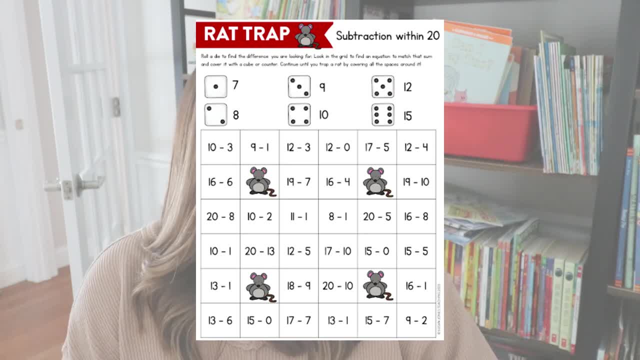 of 12.. This game is a bit more advanced, as they are matching the difference to the equation instead of, you know, looking at an equation and trying to find the difference. So this is one of the different ways that you can do this. So let me show you what it looks like in my subtraction. 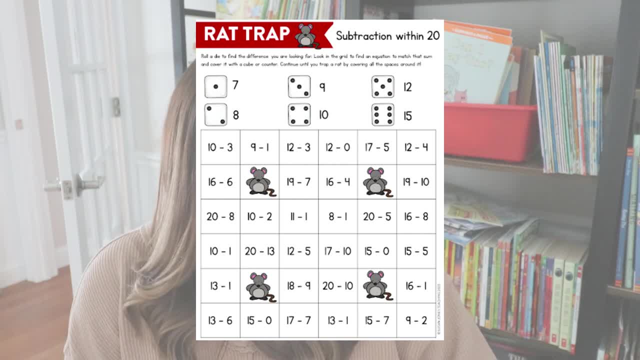 unit but all students will do is, once they find an equation that matches the difference they're looking for, they will cover it with a cube. So, for example, if they rolled a one and they're looking for a difference of seven, they could cover this 10 minus three equation over in the 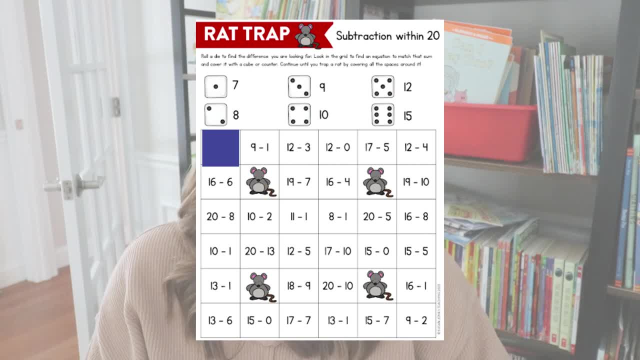 top left And they'll do that with their color cube or counter or whatever you're using. But you do want students to have different color manipulatives, Then player number two will go and let's pretend they roll a two and they're looking for a difference of eight. They could go. 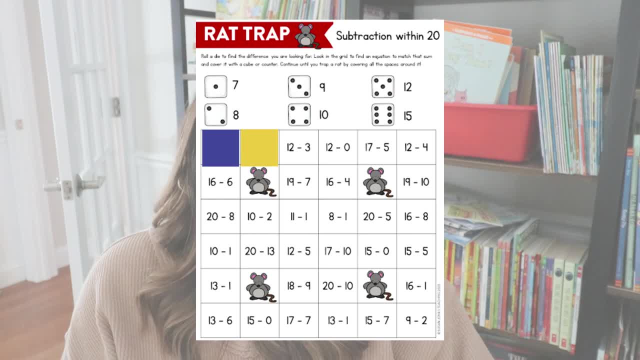 ahead and cover up that nine minus one equation, because nine minus one equals eight. Students keep rolling, finding the correct equation to match the difference and covering the boxes until they trap a rat. And the way that they actually trap a rat is by building a box around one of 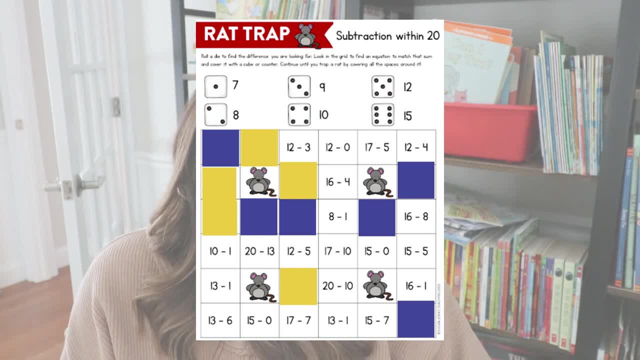 the rats, And the winner for this game would be the player who can place their last cube to trap the rat. So it doesn't matter if you both have cubes going around the rat. it's the person who gets to put the last cube there to finally. 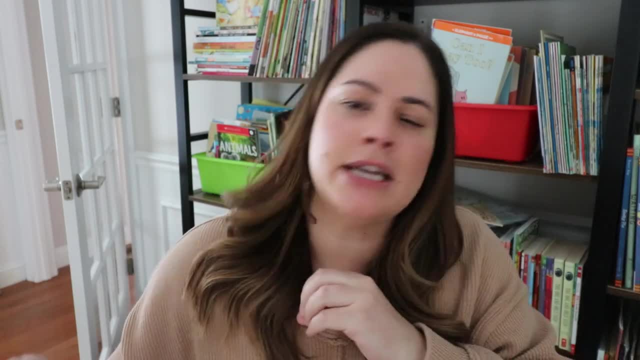 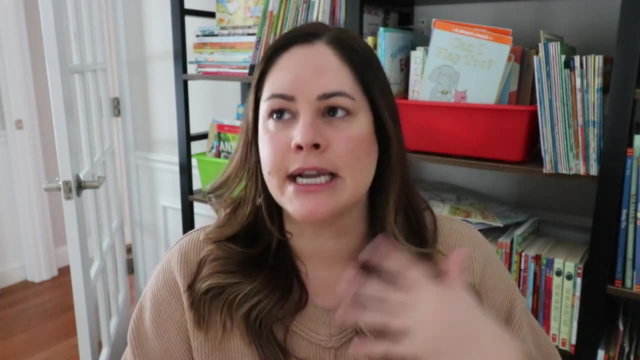 trap it, that wins the game. Like I said, that game is a little trickier because, instead of getting an equation and finding the difference, they're reversing that thinking and they have to roll the die to match the difference. So it requires a couple layers. 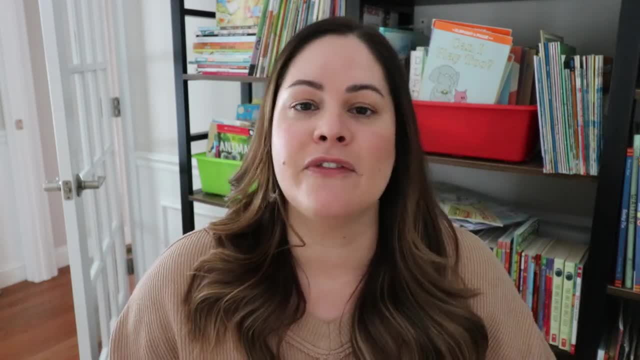 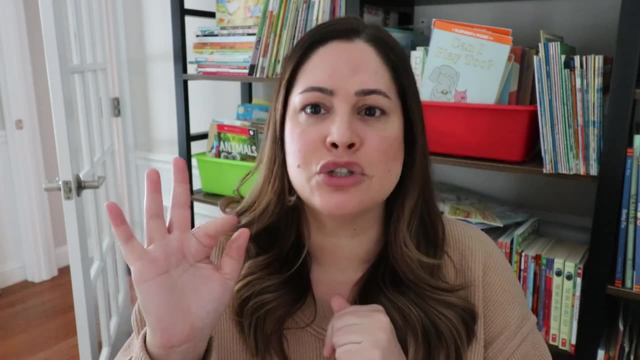 of thinking, which is great for students, but it's also a whole lot of fun seeing who can trap that rat first And, like I mentioned, I have five different boards with subtraction within different numbers: 10,, 20,, 50,, 100, and 1000.. So it really is great for kindergarten through second grade. 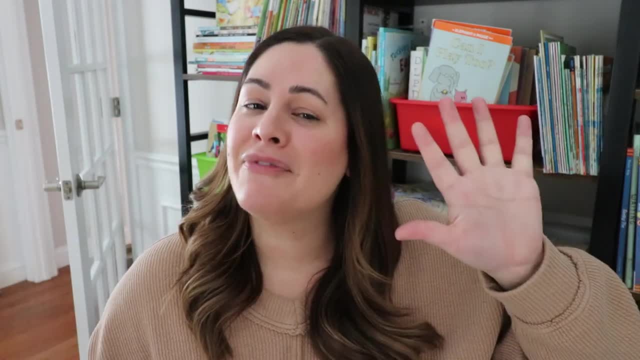 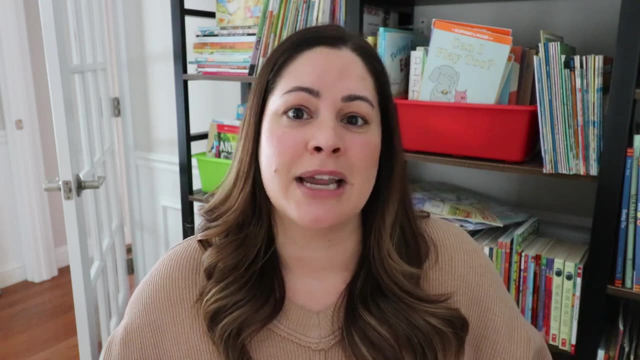 I will link that freebie down in the description as well. So there you have five of my favorite subtraction games to play in a primary classroom. I hope you can see from most of them that you can really differentiate based on the needs of your students by giving them manipulatives or scrap. 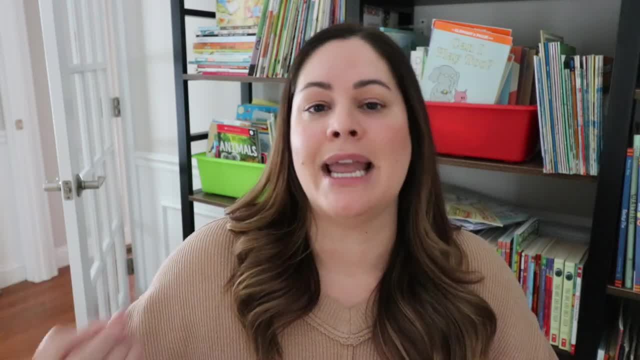 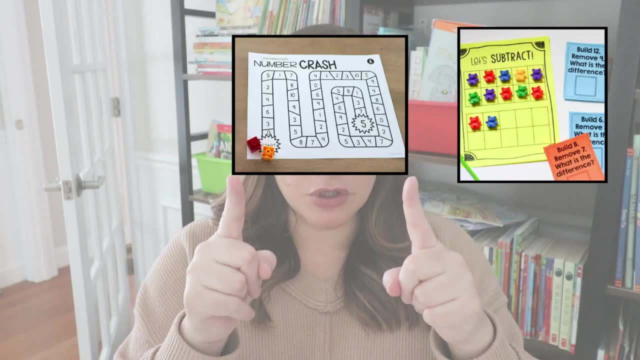 paper and then really building towards that fluency of being able to solve subtraction without those pieces. Just for a quick recap: we have build and remove, we have number crash, we have fill the spaces, we have subtraction, switcheroo or any of the. 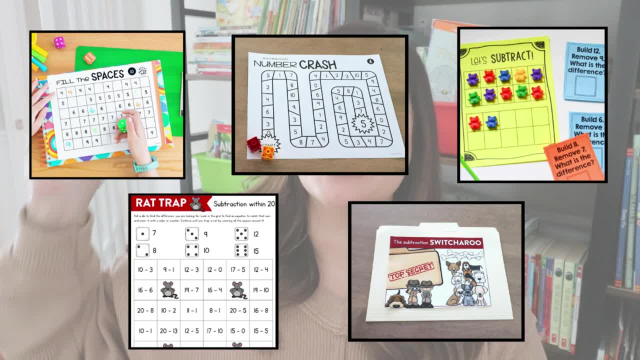 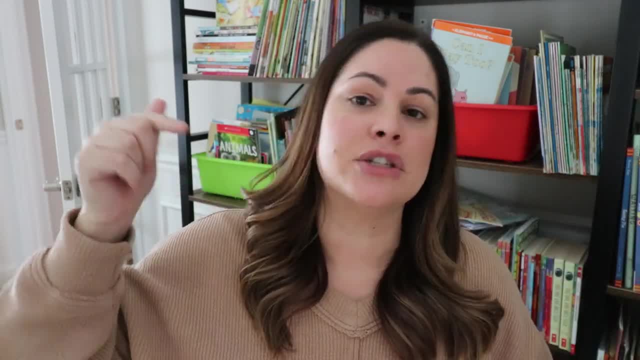 math mysteries and we have rat trap and, like i said earlier, rat trap and fill the spaces are completely free and they will be linked down in the description. i will, of course, link everything down below in the description and just so you know if you are in the sjt math club. all of these games. 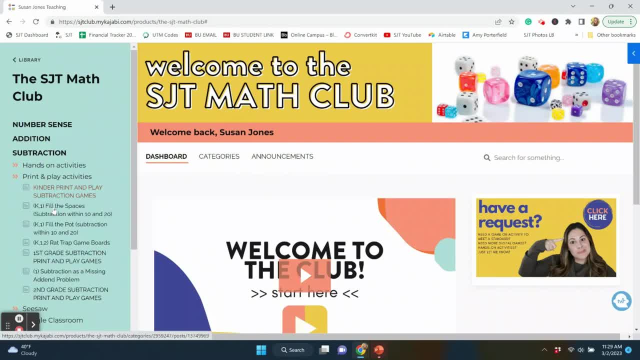 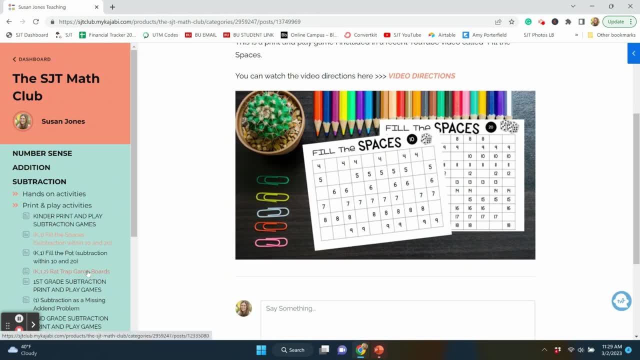 and activities are already in the club for you. if you look under the subtraction section, you will either go to hands-on games or print and play games to find what you are looking for, and if you're looking for the digital versions of the math mysteries, it's under the digital section.